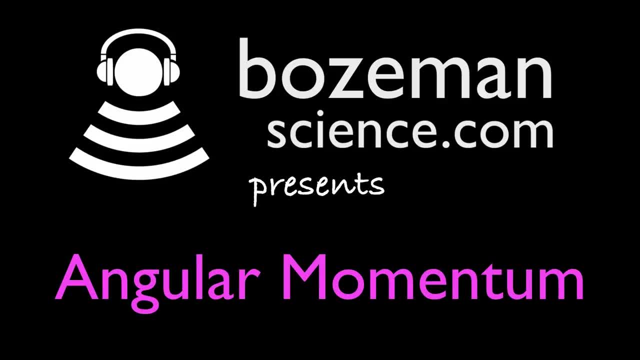 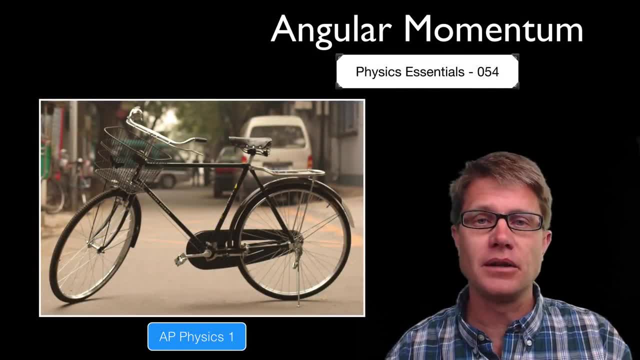 Hi, It is Mr Andersen, and this is AP Physics essentials, video 54. It is on angular momentum. Momentum, remember, is a product of the mass times, the velocity of an object. So any object moving with mass has momentum. The only difference in angular momentum is: 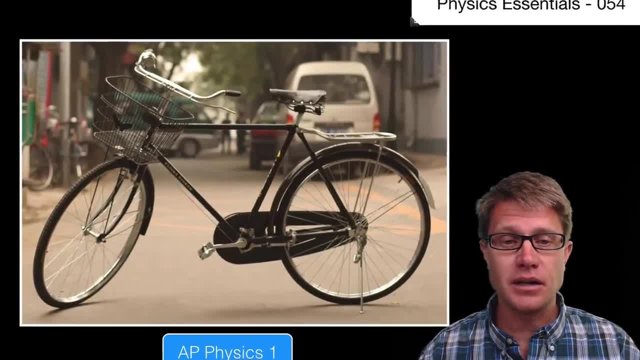 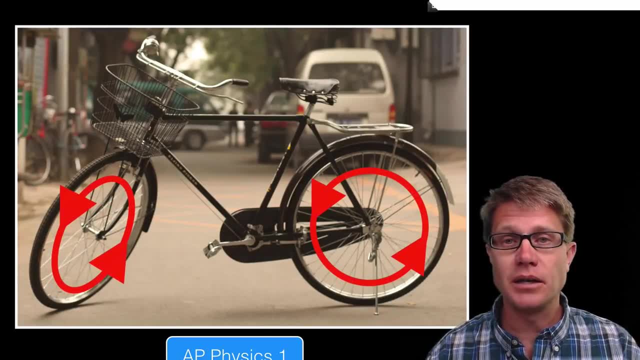 it is rotating or spinning objects, And so if you were to try to get on this bicycle and balance without the kickstand out, you are probably going to fall over. But as you start to bike, as these wheels pick up angular momentum, they are going to resist changes. 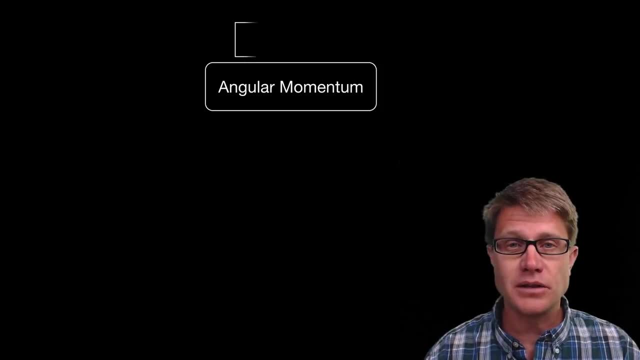 And it makes it easier for you to remain upright. And so angular momentum is a vector, And so there is a clear direction in which it acts, And in AP Physics you should be able to understand the angular momentum of either a point object. So a point object is going to be an object. 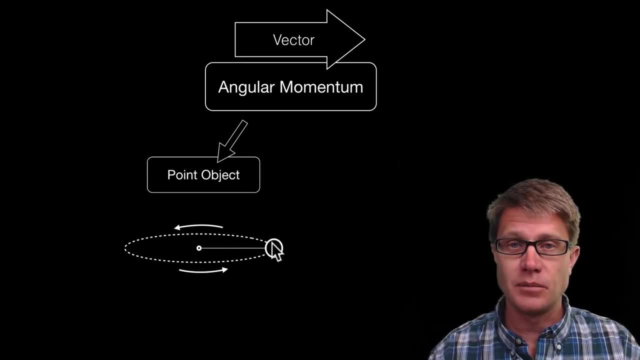 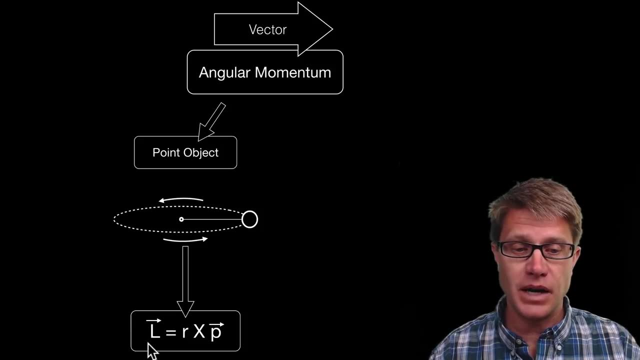 accelerating around a point, So it could be, for example, an object attached to a spring or a planet orbiting around the sun, And the equation is very simple: It is going to be equal. L is equal to our angular momentum. Again, it is a vector Which is equal to r. 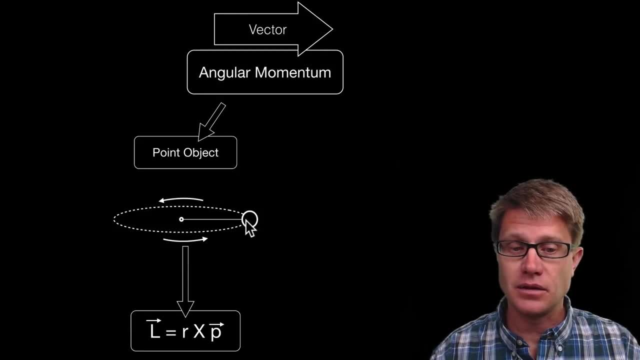 that is going to be the radius from the center to the object. So that is the distance times its linear momentum, which would be the mass times the velocity in a line. You also should be able to calculate the angular momentum of an extended object, So the whole object. 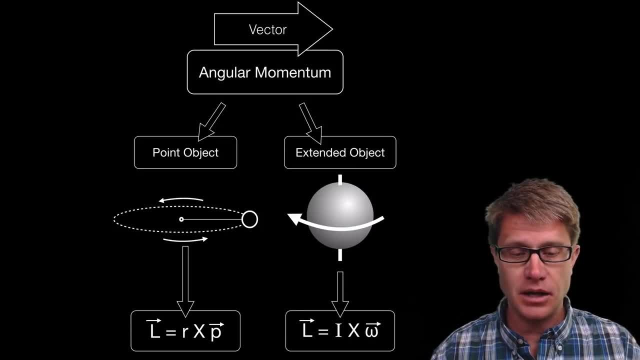 is rotating around a point. So to figure that out, all we say is that angular momentum is equal to I, where that is rotational inertia times the angular velocity. So that is the velocity of the object, And again that inertia is going to change depending on what that. 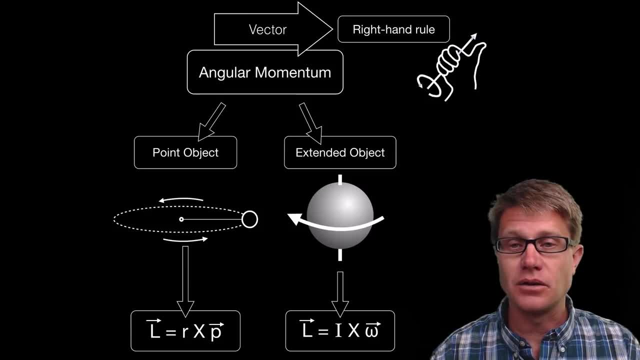 object is Now to figure out the direction of this vector, you will use the right hand rule. So if we look at this one right here, the object is spinning like that. So if you move your fingers in the direction of that spin, then we should have angular momentum. 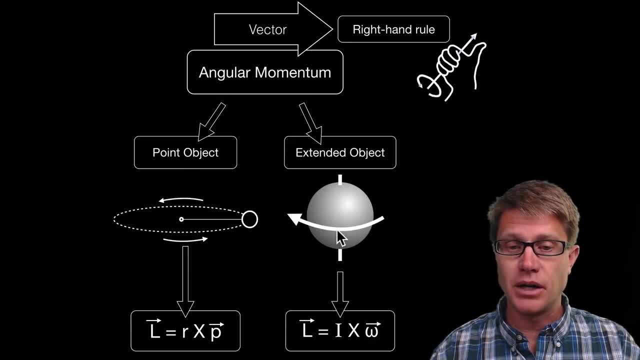 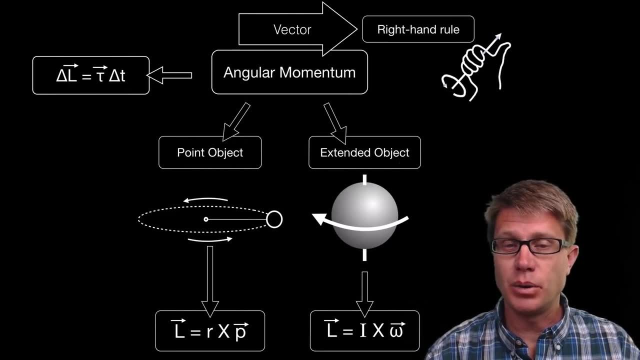 that is moving in the upward direction, Whereas on this one, since it is rotating in the other direction, we are going to have it acting in the downward direction. Now we learned when we were dealing with impulse that if you apply a force, you are going to be able to move. 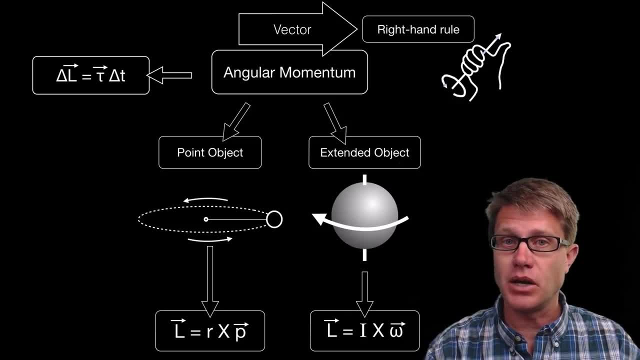 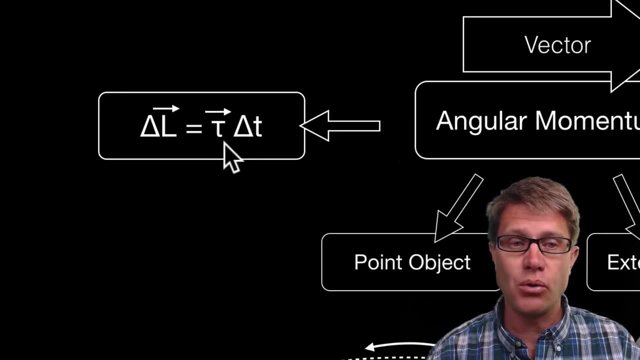 a force for a given period of time, That is going to equal the change in momentum of the object. Well, the same applies here. So the change in angular momentum is equal to not the impulse but rather the torque times, the change in time, So that net torque times. 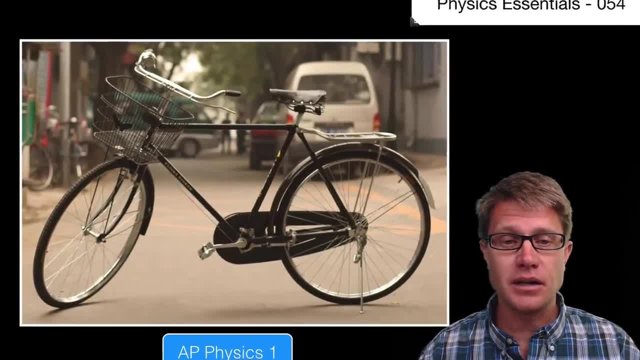 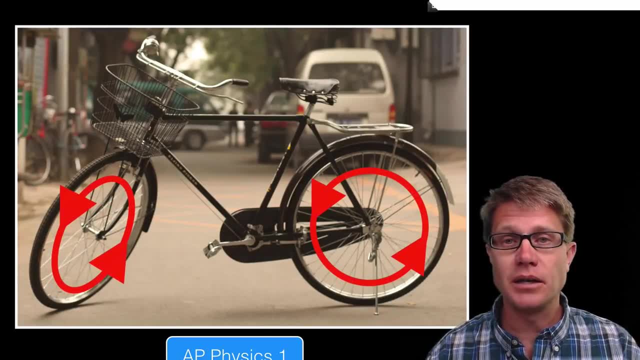 it is rotating or spinning objects, And so if you were to try to get on this bicycle and balance without the kickstand out, you are probably going to fall over. But as you start to bike, as these wheels pick up angular momentum, they are going to resist changes. 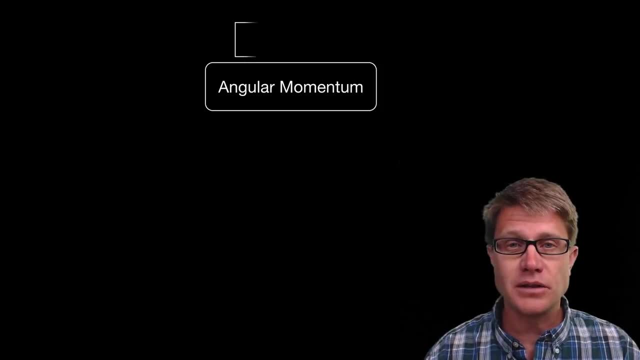 And it makes it easier for you to remain upright. And so angular momentum is a vector, And so there is a clear direction in which it acts, And in AP Physics you should be able to understand the angular momentum of either a point object. So a point object is going to be an object. 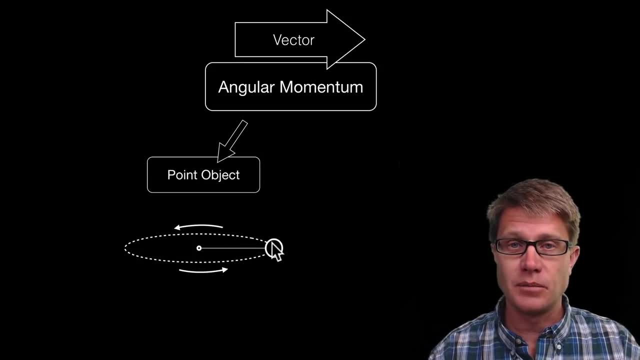 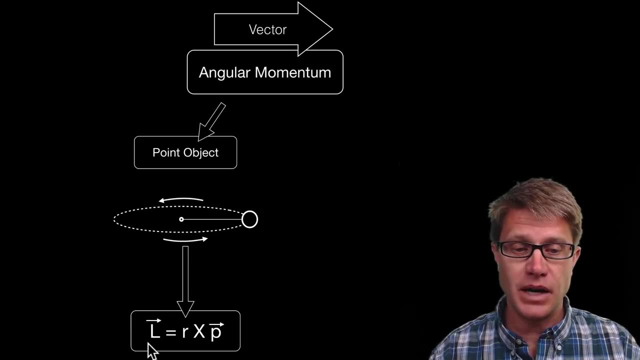 accelerating around a point, So it could be, for example, an object attached to a spring or a planet orbiting around the sun, And the equation is very simple: It is going to be equal. L is equal to our angular momentum. again, it is a vector which is equal to r. 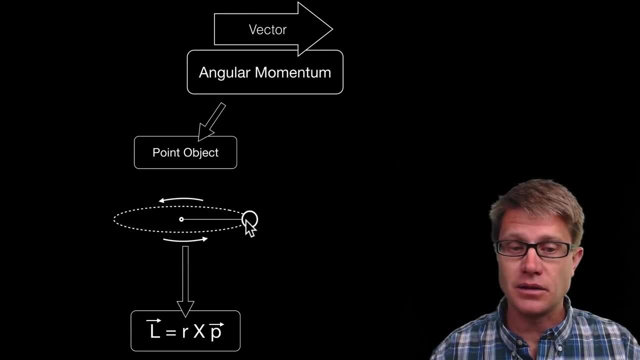 that is going to be the radius from the center to the object, so that is the distance times its linear momentum, which would be the mass times the velocity in a line. You also should be able to calculate the angular momentum of an extended object, So the whole object. 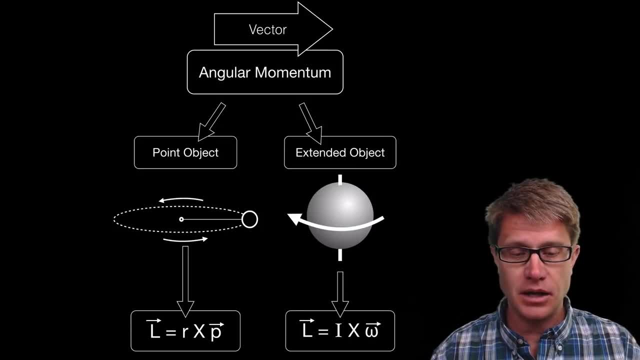 is rotating around a point. So to figure that out, all we say is that angular momentum is equal to i, where that is rotational inertia times the angular velocity, And that is the velocity of the object, And again that inertia is going to change depending on what that 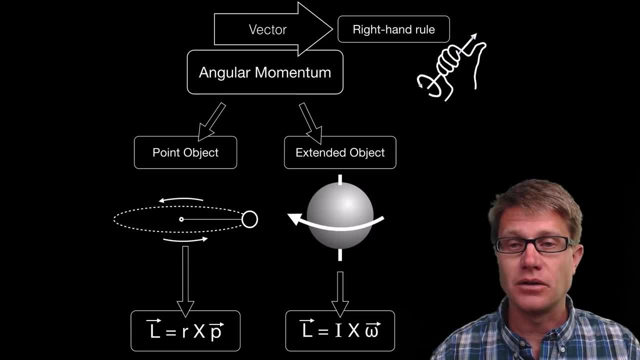 object is Now to figure out the direction of this vector, you will use the right hand rule. So if we look at this one right here, the object is spinning like that. So if you move your fingers in the direction of that spin, then we should have angular momentum. 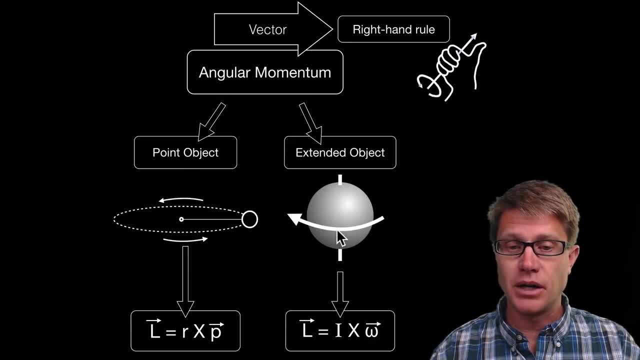 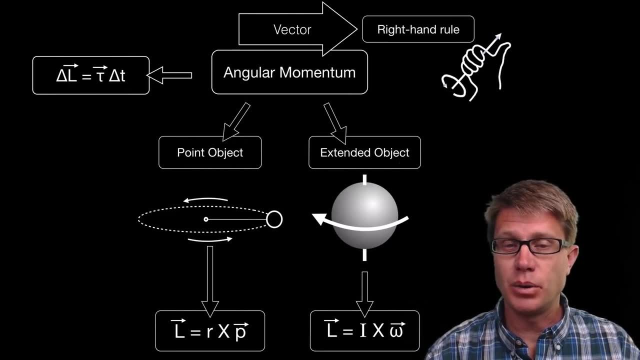 that is moving in the upward direction, Whereas on this one, since it is rotating in the other direction, we are going to have it acting in the downward direction. Now we learned when we were dealing with impulse that if you apply a force, you are going to be able to move. 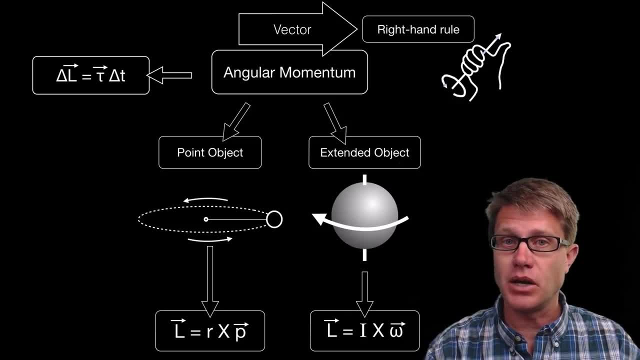 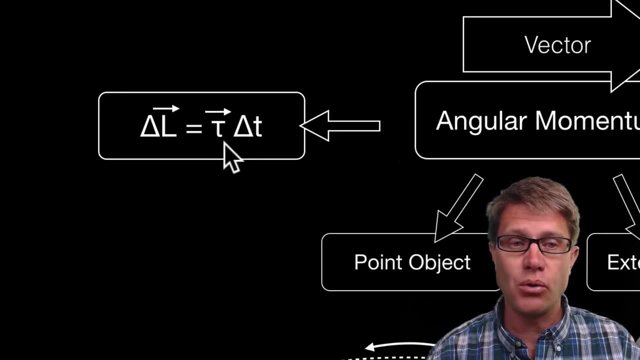 a force for a given period of time, That is going to equal the change in momentum of the object. Well, the same applies here. So the change in angular momentum is equal to not the impulse but rather the torque times, the change in time, So that net torque times. 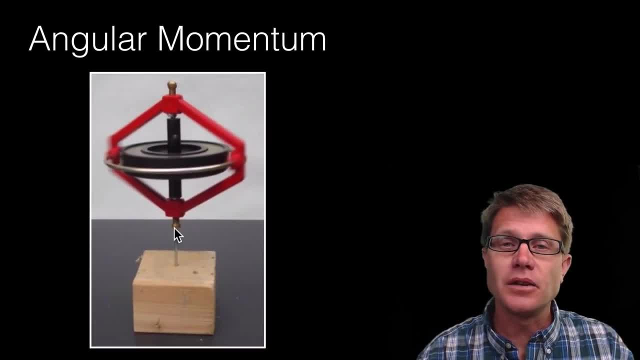 the change in time is going to give us a change in that angular momentum. So angular momentum of this gyroscope, since we are spinning it in this plane, that is going to keep it spinning in that plane, And so it is able to resist changes due to gravity. There are really neat. 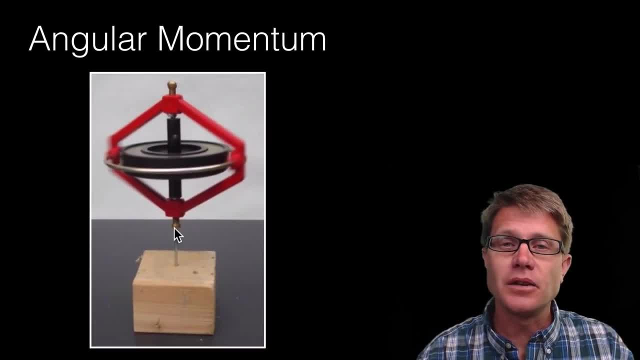 the change in time is going to give us a change in that angular momentum. So angular momentum of this gyroscope, since we are spinning it in this plane, that is going to keep it spinning in that plane, And so it is able to resist changes due to gravity. There are really neat. 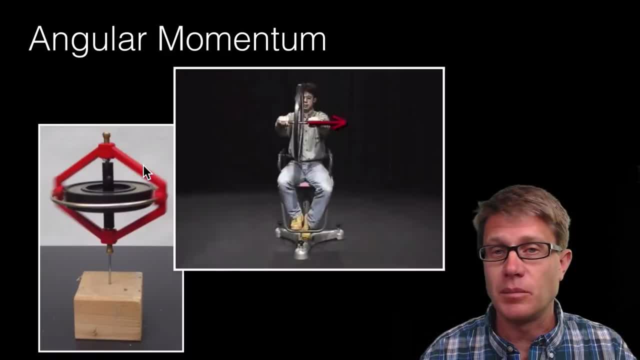 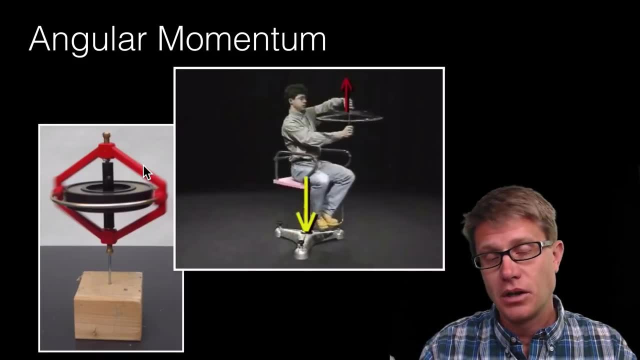 things we will do in future videos. So you can take a wheel and give it a spin, You can give it a certain amount of angular momentum, like that, And so it is conserved. but it can be transferred, some of that angular momentum, as we change the angle at which that force. 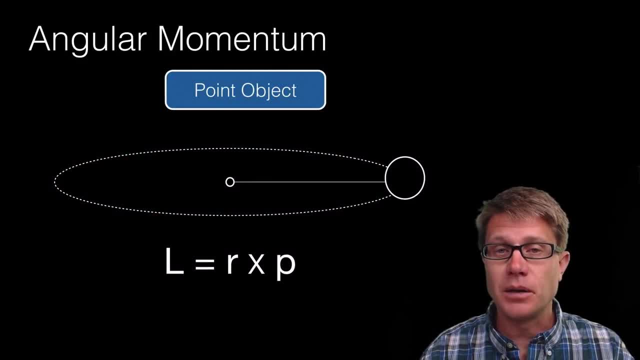 is actually acting, And so the two things you should be able to do in AP physics is calculate the angular momentum of a point object. Again, that is an object that is moving or rotating around a given point, So this could be an object attached to a string, or 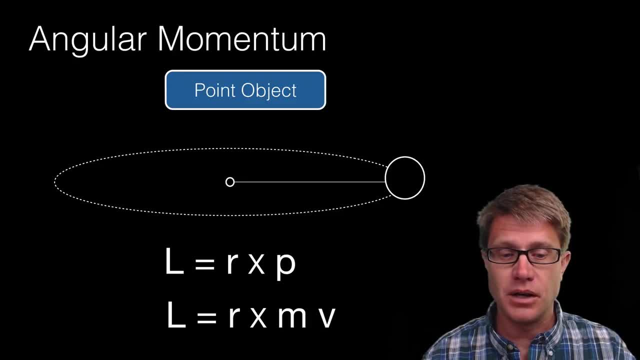 the moon orbiting around the earth, And so the formula is pretty easy. It is simply r, which is the radial distance, And that is the angular momentum of the force. So that is the angular momentum of the force. So the formula is pretty easy. It is simply r, which is the radial 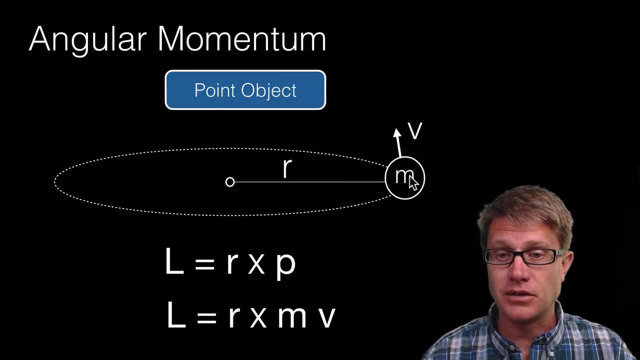 distance here times the linear momentum. So linear momentum is going to be in this direction. So it is the mass times the velocity. And so if you have these three bits of information- the velocity of the object, the mass and the radius- all we do is simply multiply those. 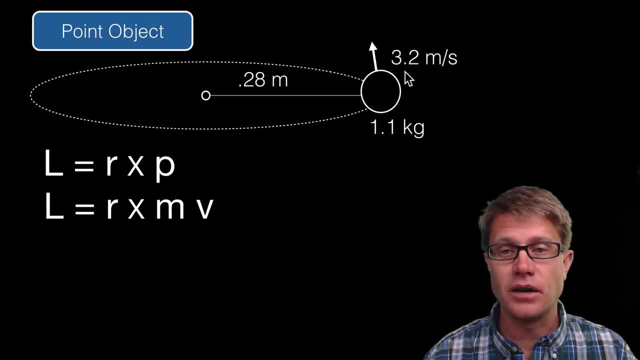 together. So let's say we had an object- 1.1 kilogram mass- traveling at 3.2 meters per second, And then we have got about 28 centimeters here distance between the two. All we are going to do is multiply those values out And then we are going to get an angular momentum. 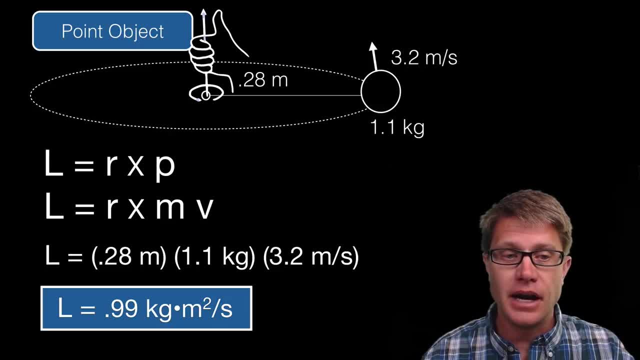 of 0.99 kilogram meters squared per second. Now, the one thing I should have included here is that this is a vector value, So we have to add a direction to it. How do we figure out the direction? Well, since the rotation is like this, we use the right hand rule to. 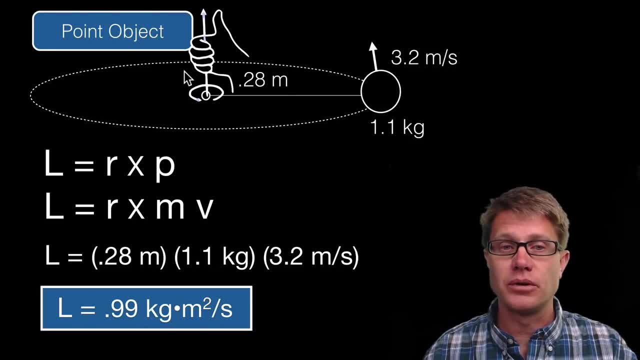 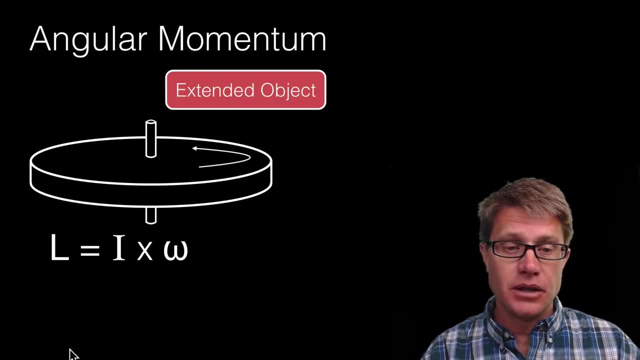 show that that angular momentum is going to be acting in the upward direction. You also should be able to calculate the angular momentum of an extended object like this rotating cylinder. here All we do is multiply the rotational inertia times the angular velocity of that object. So if it is given, let's say we have an inertia of 15 kilogram meters. 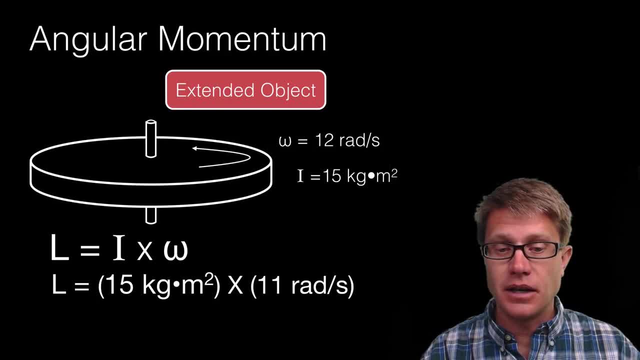 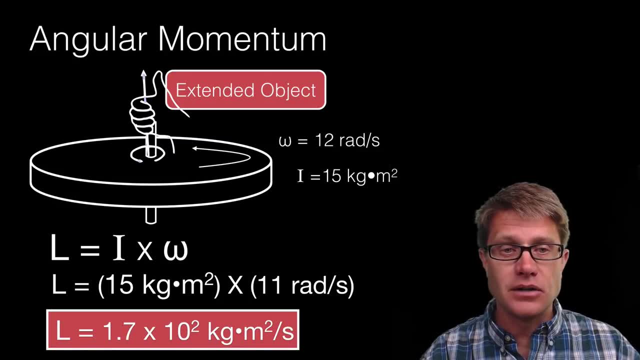 squared. We multiply that times our angular velocity like that And we are going to get 1.7 times 10 to the second kilogram meters squared per second. Now, this again is a vector, And so what direction is that acting? Again, looking at my right hand rule, it is going. 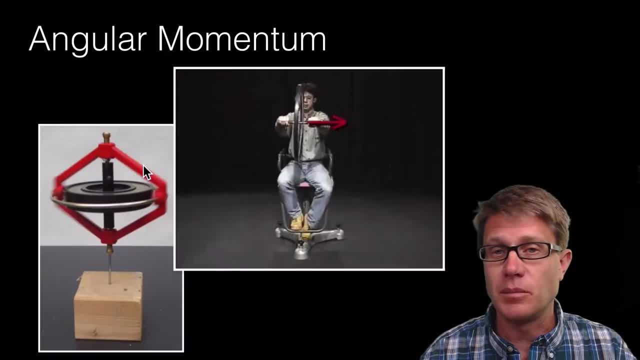 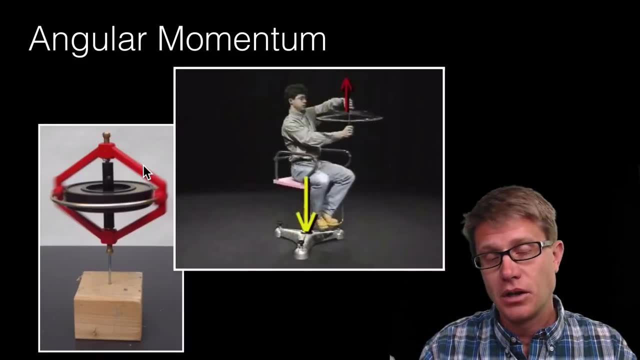 things we will do in future videos. So you can take a wheel and give it a spin, You can wheel and give it a certain amount of angular momentum, like that, And so it is conserved. but it can be transferred, some of that angular momentum, as we change the angle at which that 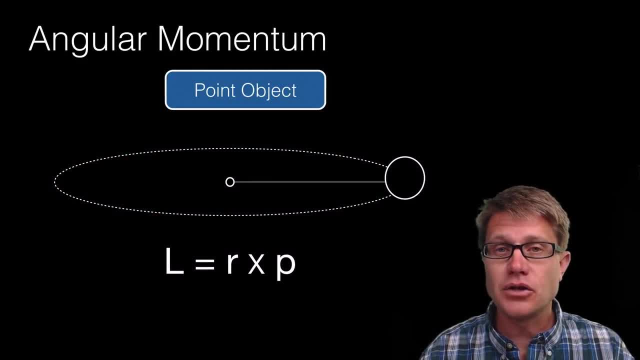 force is actually acting, And so the two things you should be able to do in AP physics is calculate the angular momentum of a point object. Again, that is, an object that is moving or rotating around a given point, So this could be an object attached to a string, or 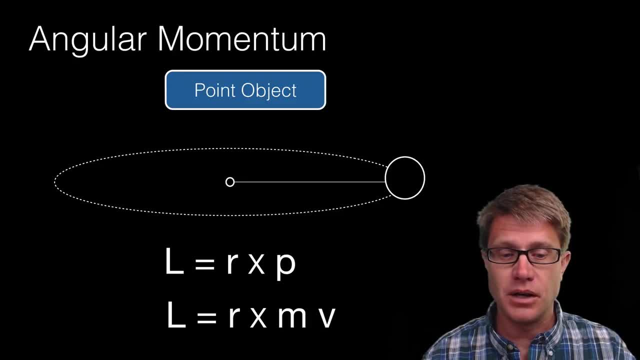 the moon orbiting around the earth, And so the formula is pretty easy. It is simply r, which is the radial distance here times the linear momentum. So linear momentum is going to be in this direction. So it is the mass times the velocity, And so, if you have these, 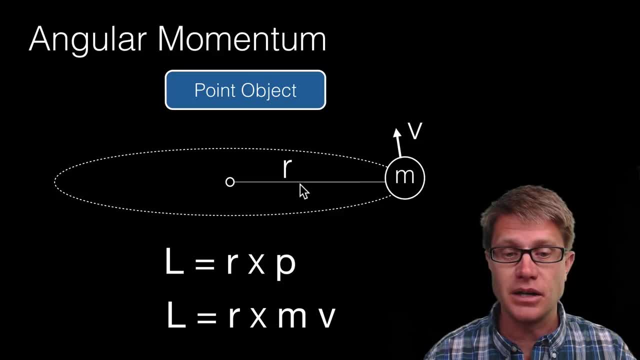 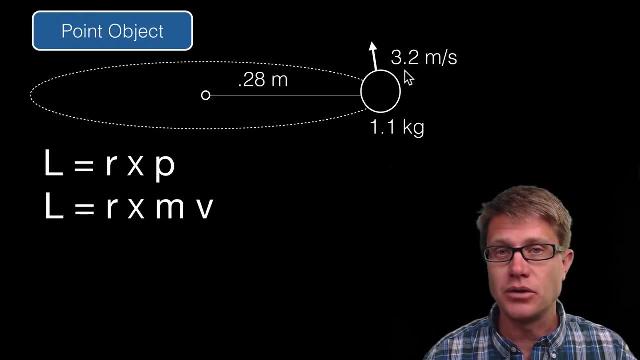 three bits of information: the velocity of the object, the mass and the radius. all we do is simply multiply those together. So let's say we had an object, 1.1 kilogram mass, traveling at 3.2 meters per second, And then we have got about 28 centimeter here, distance between 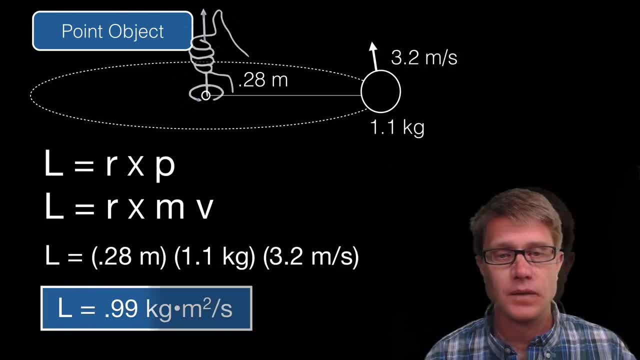 the two. All we are going to do is multiply those values out, And then we are going to calculate the angular momentum of 0.99 kilogram meters squared per second. Now, the one thing I should have included here is that this is a vector value, So we have to add a direction. 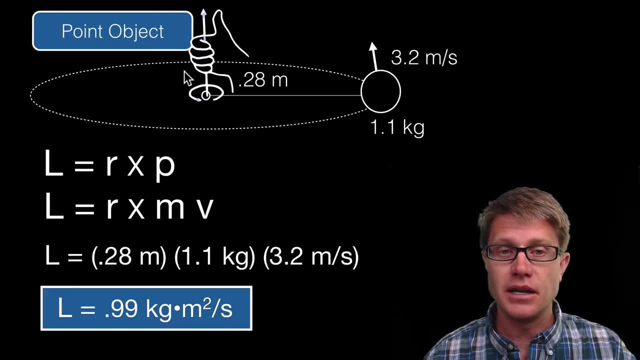 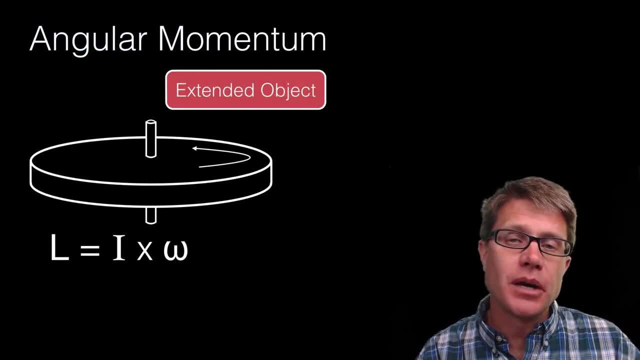 to it. How do we figure out the direction? Well, since the rotation is like this, we use the right hand rule to show that that angular momentum is going to be acting in the upward direction. You also should be able to calculate the angular momentum of an extended object. 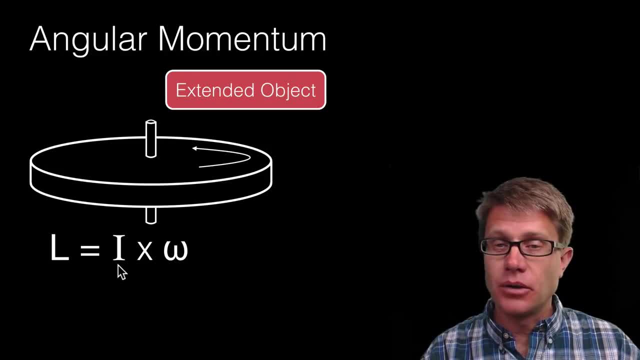 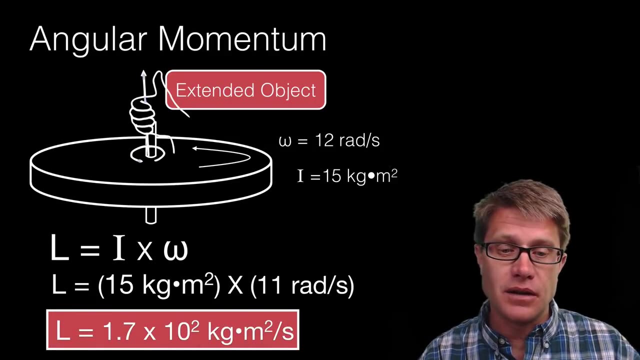 like this rotating cylinder. here All we do is multiply the rotational inertia times the angular velocity. So if it is given, let's say, we have an inertia of 15 kilogram meters squared, We multiply that times our angular velocity, like that And we are going to get 1.7 times 10 to the 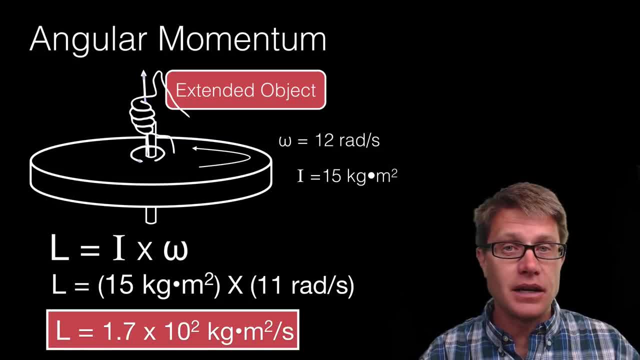 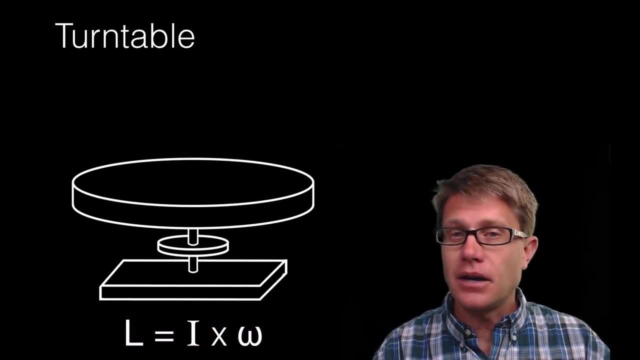 second, kilogram meters squared per second. Now, this again is a vector, And so what direction is that acting? Again, looking at my right hand rule, it is going to be acting in the upward direction. Now, how do we measure this in the physics lab? A good way to play around. 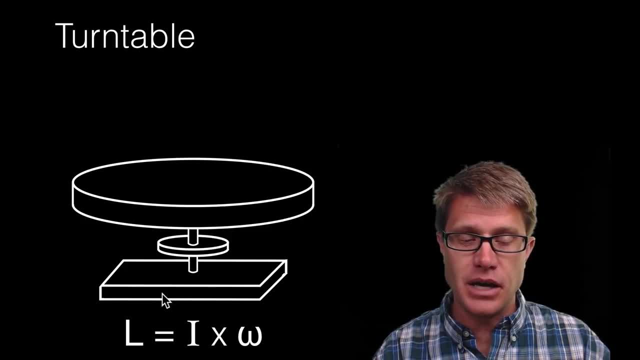 with this is using a turntable. So you can use a turntable that is attached to a desk. It has a certain amount of mass on it And what you can do is you can give it a spin. So if we spin it in that direction we try to make, 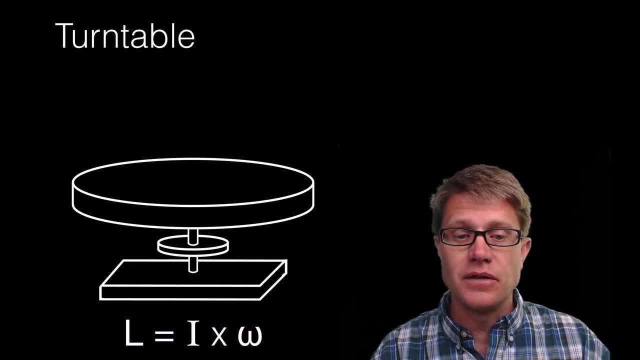 to be acting in the upward direction. Now, how do we measure this in the physics lab? A good way to play around with this is using a turntable. So you can use a turntable that is attached to a desk. It has a certain amount of mass on it And what you can do is you. 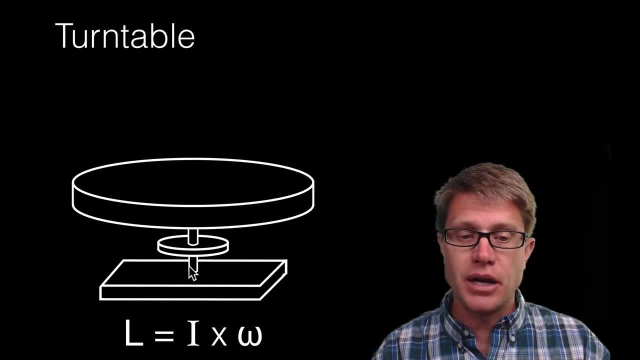 can give it a spin. So if we spin it in that direction, we try to make it as frictionless as we can. it is just going to keep spinning in that direction And these are generally pretty heavy, So they have a large amount of rotational inertia. You can also attach. 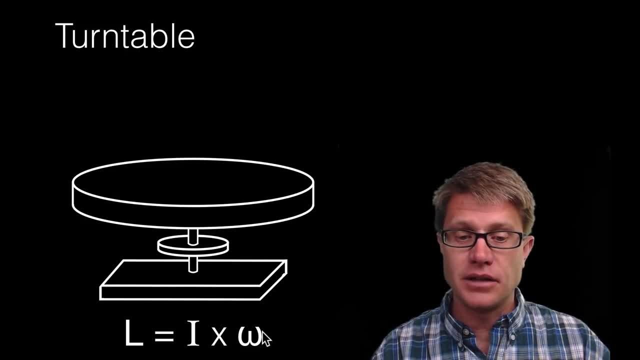 a photogate to it so we can measure that angular velocity or the speed at which it is turning in radians per second, And so you can do calculations of rotational inertia. We can also do collisions. Let's say we were to take another object, As the bottom object is spinning with a certain 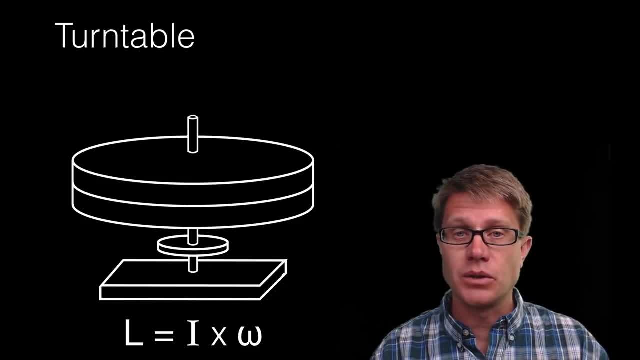 angular velocity, we could simply drop the rotation, And that is what we are going to do with the top object on it. So what is going to happen is the angular momentum is going to be conserved, And so we are going to have to see a decrease when we put both of these. 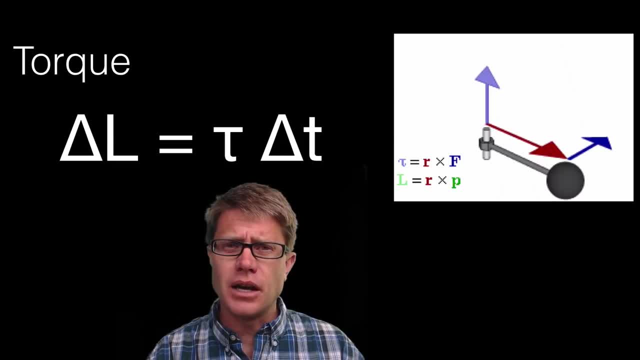 together in its angular velocity. Also, you should understand how a change in torque or net torque over a given period of time is going to change the angular momentum. This is just like impulse in regular translational motion. And so here we have got an object. 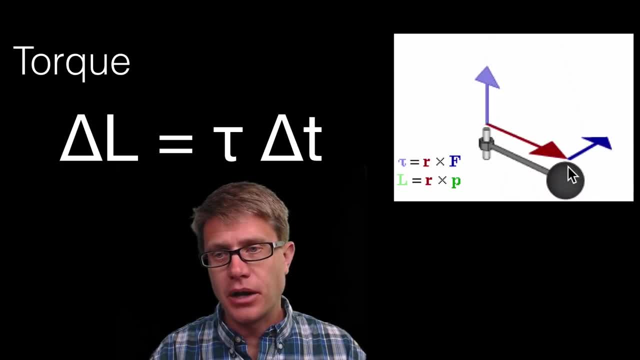 and we are going to apply a force to it in this direction. Remember, if we apply a force perpendicular to the lever arm, we are going to get a torque, And so the torque is going to be in this direction. So I am going to start the animation and watch. 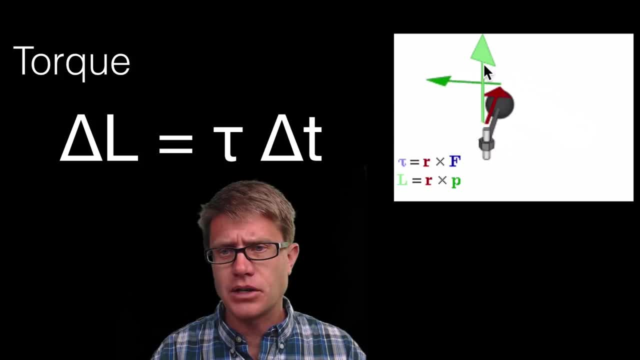 what happens to the angular momentum. So as I add a force in that direction, we are getting an angular momentum in this direction. What is causing that angular momentum? Again, it is the lever arm now times the momentum in that direction. So as we apply a torque, it. 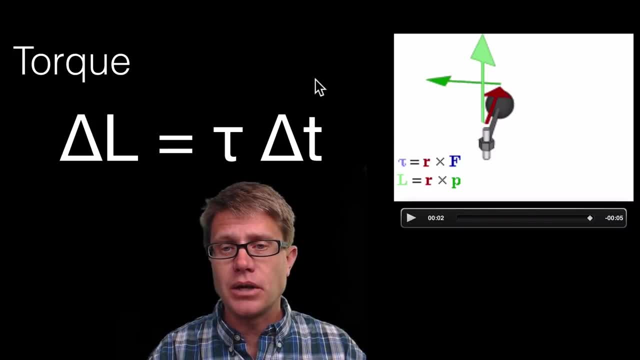 takes a while, but we are building up momentum in that direction. Now watch what happens if we change the torque in the other direction. So again, it already has some movement or momentum in this direction, But now we have reversed the torque So it is going to be applying a force in this direction. 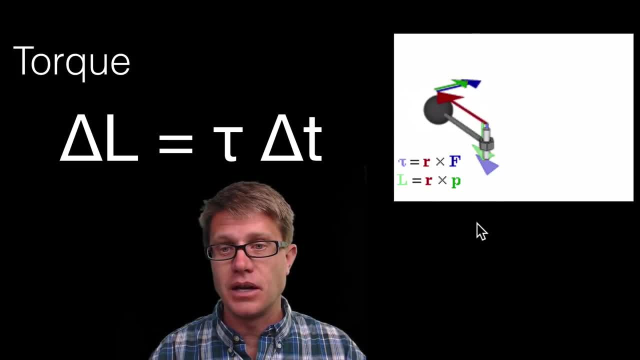 So the torque is down. Watch what happens. We are going to see a decrease in angular momentum and then it goes in the other direction. And so again, as we apply a torque against that angular momentum, what do we get? At this point, we can bring it to a stand still. 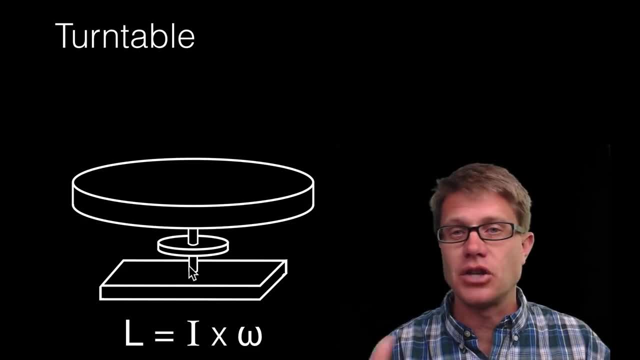 it as frictionless as we can. it is just going to keep spinning in that direction, And these are generally pretty heavy, So they have a large amount of rotational inertia. You can also attach a photogate to it so we can measure that angular velocity or the speed at which. 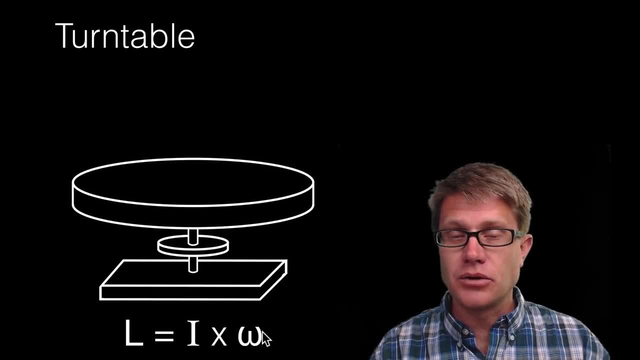 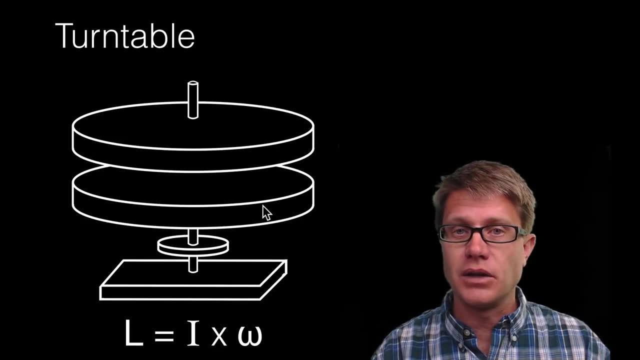 it is turning in radians per second, And so you can do calculations of rotational inertia. We can also do collisions. Let's say we were to take another object. As the bottom object is spinning with a certain angular velocity, we could simply drop the top object on it. So what is going to happen is the angular momentum is going to. 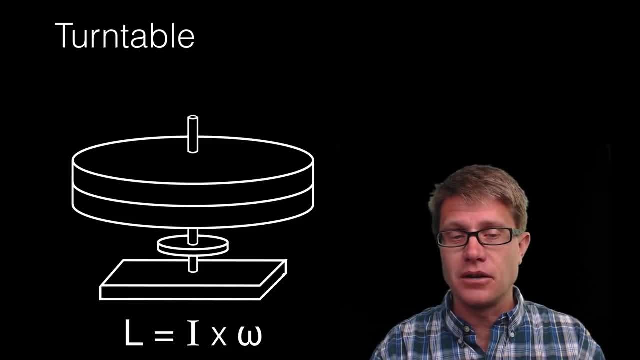 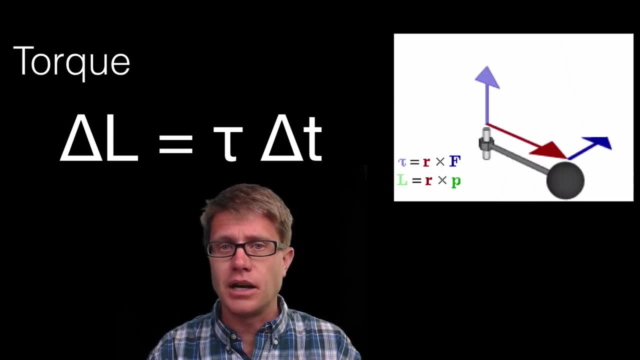 be conserved, And so we are going to have to see a decrease, when we put both of these together, in its angular velocity. Also, you should understand how a change in torque or net torque over a given period of time is going to change the angular momentum. This 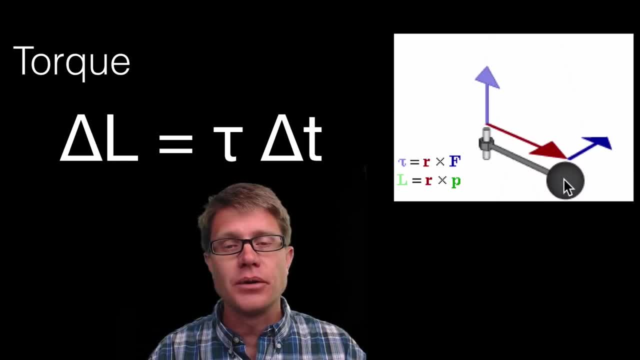 is just like impulse in regular translational motion. And so here we have got an object and we are going to apply a force to it in this direction. Remember, if we apply a force perpendicular to the lever arm, we are going to get a torque. So we are going to get a torque. 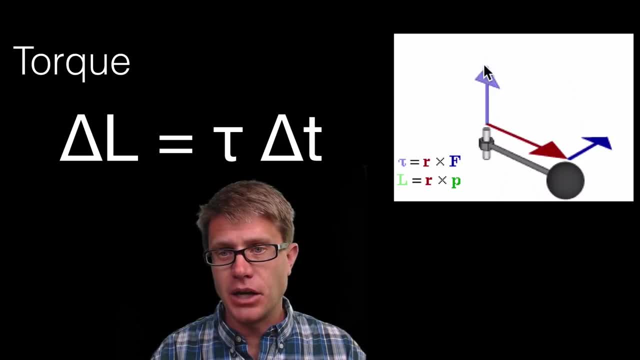 So we are going to apply a force perpendicular to the lever arm. we are going to get a torque, And so the torque is going to be in this direction. So I am going to start the animation and watch what happens to the angular momentum. So, as I add a force in that direction, we are getting 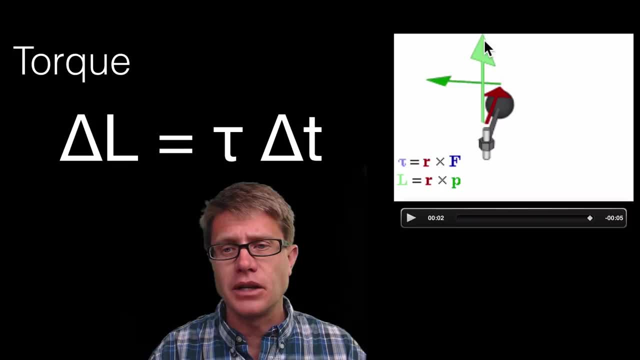 an angular momentum in this direction. What is causing that angular momentum? Again, it is the lever arm now times the momentum in that direction. So as we apply a torque, it takes a while, but we are building up momentum in that direction. Now watch what happens. 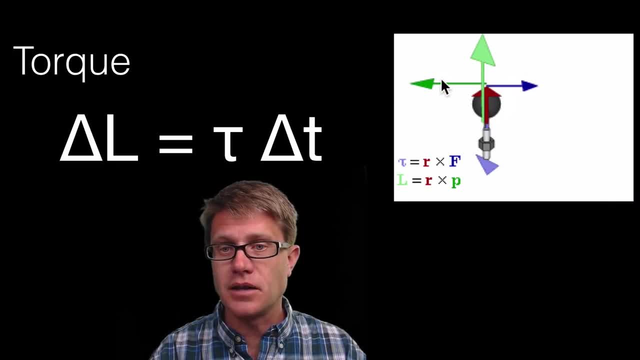 if we change the torque in the other direction. So again it already has some movement or momentum in this direction. But now we have reversed the torque So it is going to be applying a force in this direction. so the torque is down. Watch what happens. We are going to see a decrease in angular 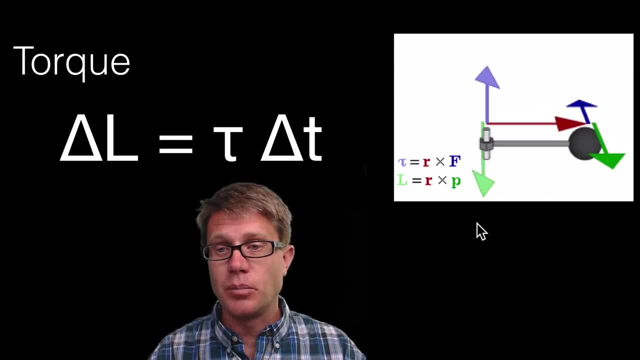 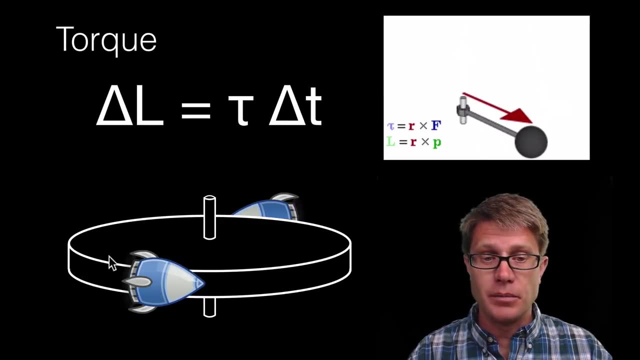 momentum, and then it goes in the other direction. And so again, as we apply a torque against that angular momentum, what do we get? At this point, we can bring it to a standstill like that. So how could we model this? Well, imagine we have this turntable right here. 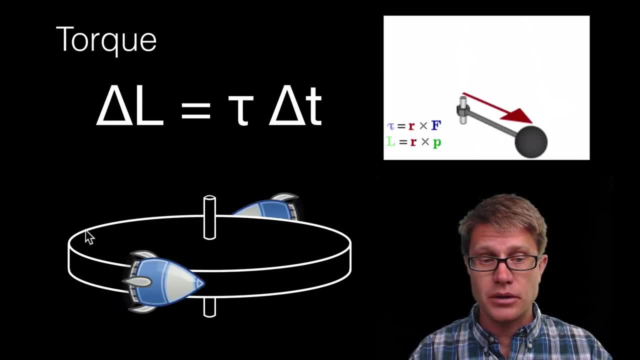 and I had rockets on either side, And they are going to apply a torque. So they are going to apply a force perpendicular to the lever arm And as they do that, over time, what is going to happen to the angular momentum? it is going to start to speed up in that direction. Now, how could 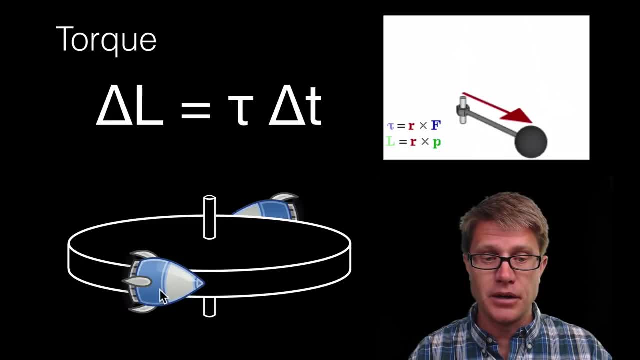 like that. So how could we model this? Well, imagine, we have this turntable right here and I had rockets on either side, And they are going to apply a torque, So they are going to apply a force perpendicular to the lever arm And as they do that over time, what is? 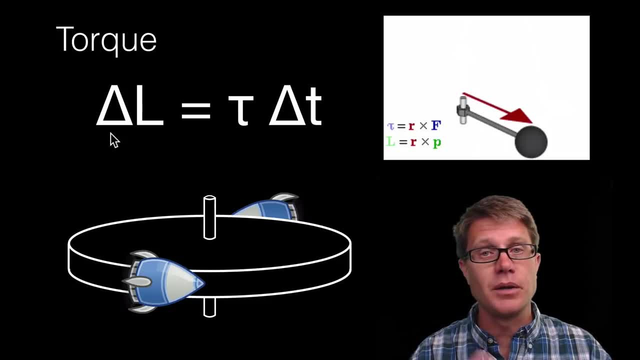 going to happen to the torque. Well, there is a torque that is going to be applied to the angular momentum. It is going to start to speed up in that direction. Now, how could you actually measure that without using rockets? You could use a setup like this. So we are. 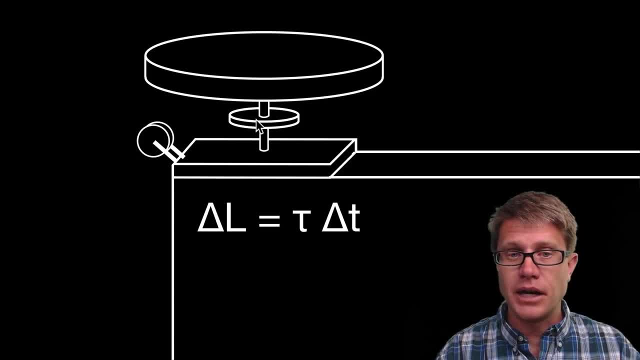 using that turntable again, We could have a little bit of a wheel down on the bottom where we can apply a force to it, And so I am having an object go off the table. Now we can apply a constant force in this direction, So that is going to be a torque over a given 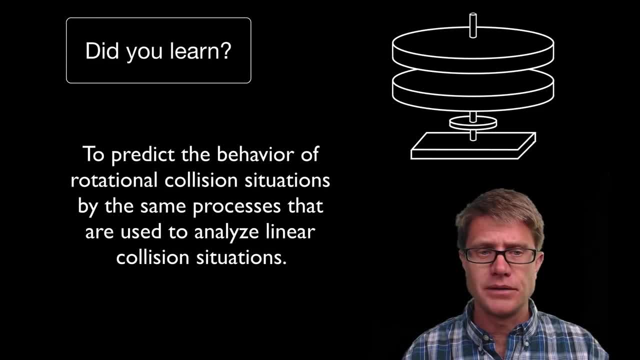 period of time, And that is going to give me my change in angular momentum. So did you learn to predict the behavior of objects in a collision as they conserve momentum? Well, I have learned to predict the behavior of objects in a collision as they conserve angular. 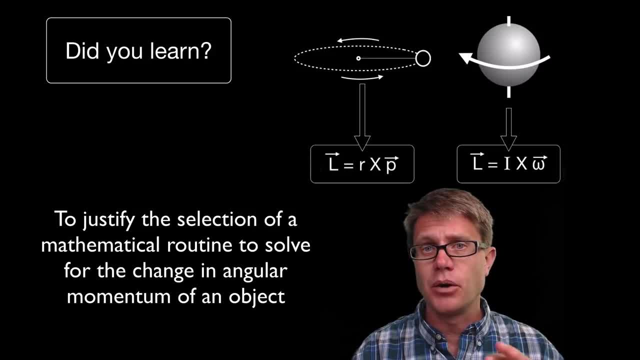 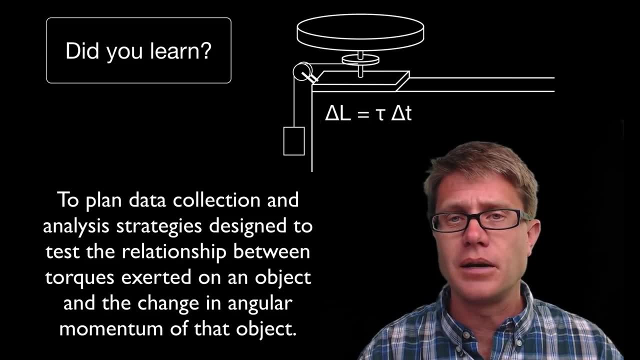 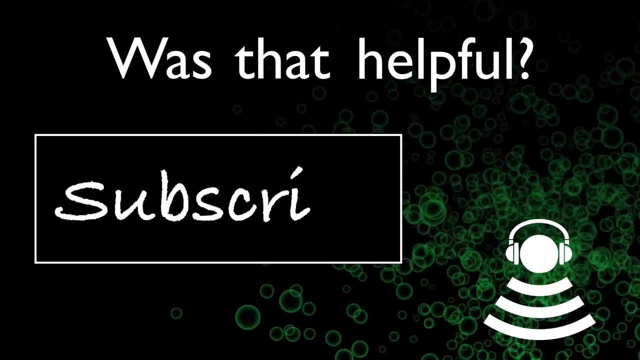 momentum. Could you calculate the angular momentum of both a point object and an extended object And also could you use torques and changing torques to see how that impacts the angular momentum of the object? I hope so And I hope that was helpful. Thank you. 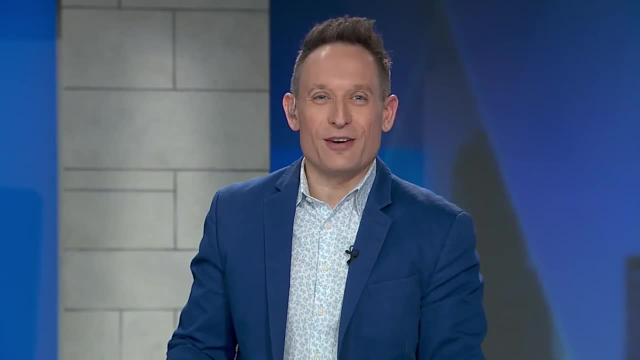 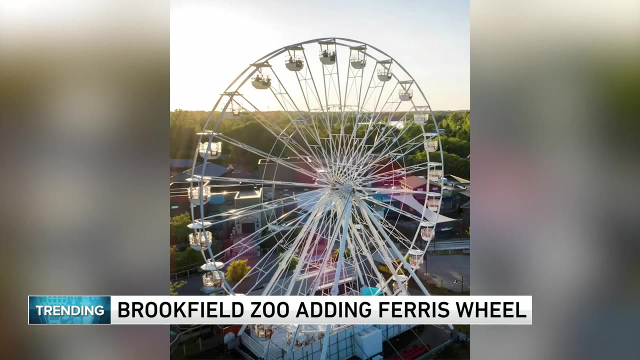 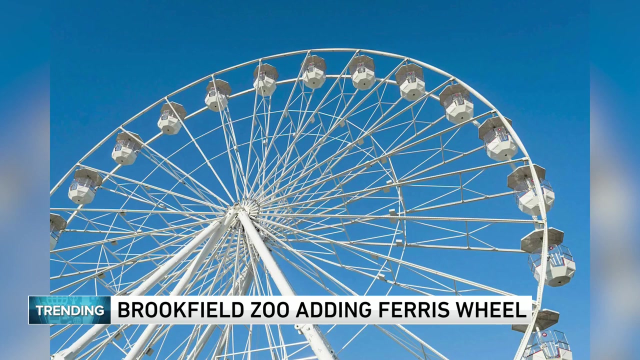 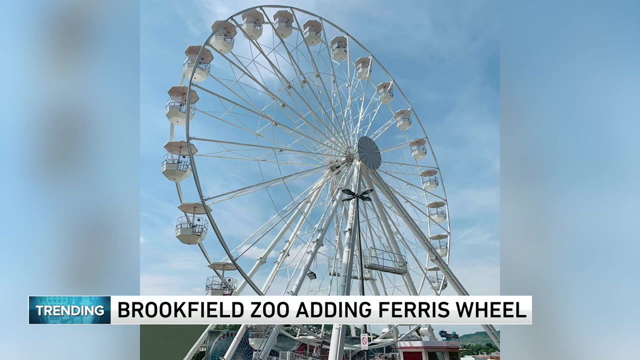 And Brookfield Zoo has announced some new attractions and events starting this spring. They include a new Ferris wheel. The ride will be 130 feet tall, feature 24 gondolas can seat six people, offering a unique view of all of the zoo's animal habitats. There'll be an extra charge for the ride: eight bucks a person, six dollars if you're a zoo member. Zoo also opening a new aviary in June will feature sandhill cranes and a dozen prairie chickens. They should put the chickens with you in the gondola while you're on the Ferris wheel. How about that? That would be fun. There you go. 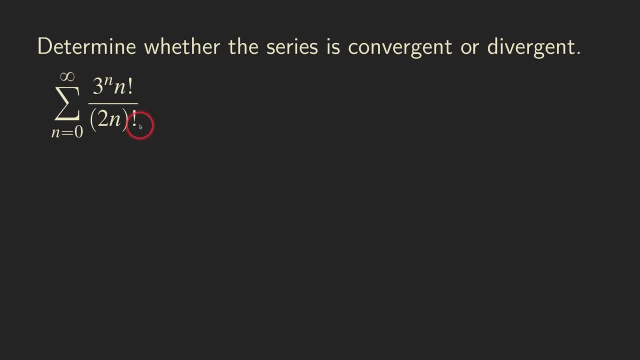 Hello everyone. Let's look at this series right here. We have a lot of factorial in there- actually just two. Okay, so to test this series for convergence, we are going to use the ratio test, And so we start by writing down the a- n turn, which is actually just this general form. 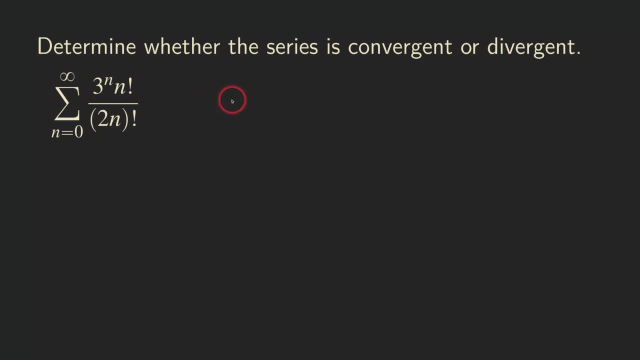 for the series, And then we also need to write down the next turn, which is the ace of n plus one turn, And then we want to take the limit of their ratio. Okay, so first we are going to just write down the ace of n turn, which is actually just this turn, right? So there's just whatever.